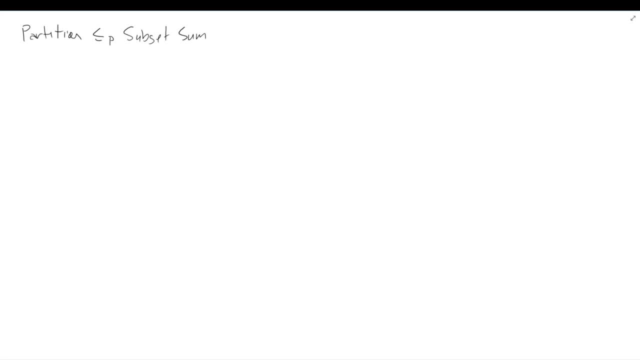 Alright, welcome. In this video I want to continue taking a look at reductions, but specifically I want to look at reductions between two problems here: partition and subset sum. Now, partition and subset sum are two problems that we've looked at in some detail already. Please refer to one of our earlier videos on NP verifiers to look at more detail about these problems. 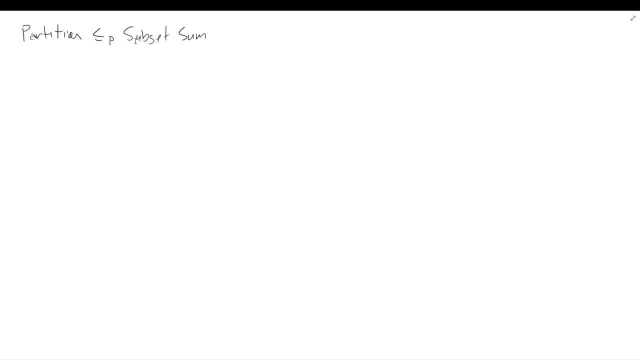 But what I want to do is show how these problems relate to each other and, in fact, this first reduction I want to take a look at. I actually want to do it in both directions, so maybe I'll do the other one over here. 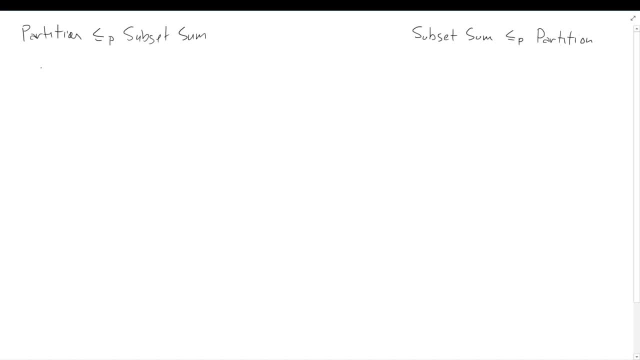 Now, if we're going to come up with these two reductions, in both cases we're going to have to come up with a mapping. So maybe I'll start that mapping off Now. in this case, we're going to start with inputs to partition. Now partition just takes a set. 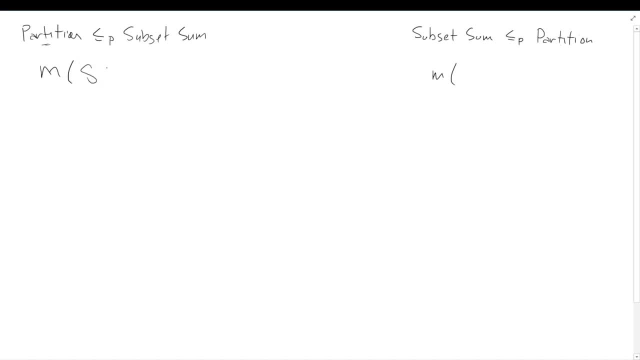 A set, A set of numbers, so maybe I'll just call that S. But subset sum takes a set and a T. Now that also sets up for what we want to return. So return: in this case we need to return an input to subset sum, which will be an S prime, and I'll call it T prime down here, but up here we just need to return an input to partition. 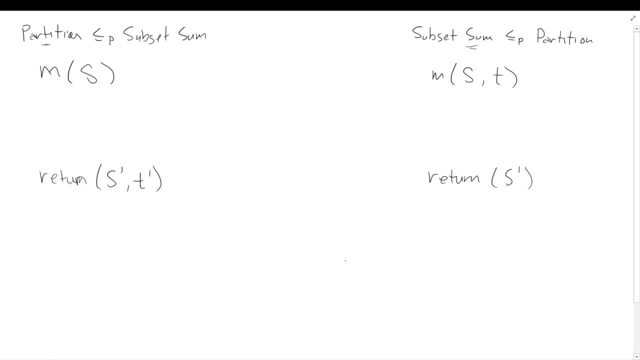 Okay, Which is just an S prime by itself. So the challenge in this reduction now remember both of these problems. ask similar questions of the input Subset. sum says: can we find a subset that adds up to T? And partition says: can we find a subset that's equal to the? that sum is equal to the sum of those left out of the subset, so the alternate set. 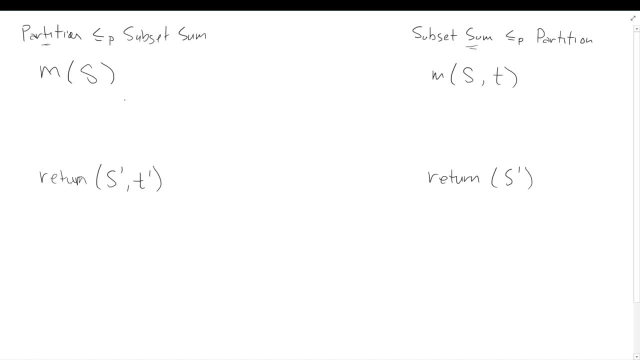 So can we partition it into two subsets with equal sum, Because both of them are asking about sums. that's not the answer. That's not the answer. They're asking about sums. that's the closely related nature. But in this direction, what we have to do is create a target sum, and that might be easy. 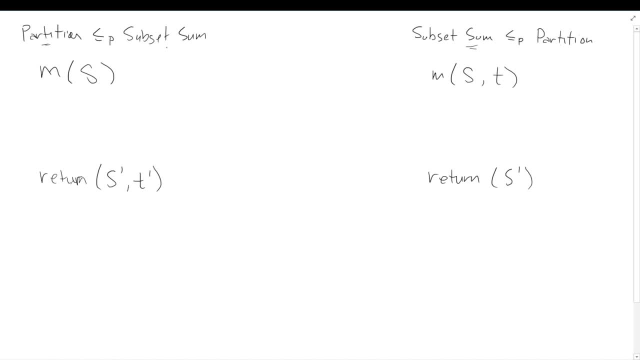 Actually, let's focus in on this. already We've already seen that in. if we're trying to do the partition problem, that's the problem where we've got this S here. Now what we could do is we could add up all the S's in S and in fact, if we took half of that, 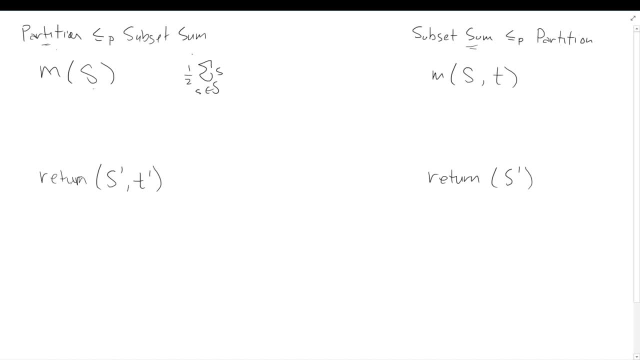 that's how much and that's how much the subset will sum to if we can equally partition it. So here in this reduction, I'm not going to change S at all. I'm going to say let S prime be equal to S, but I'm just going to go ahead and say my T prime then should be equal to this value here. 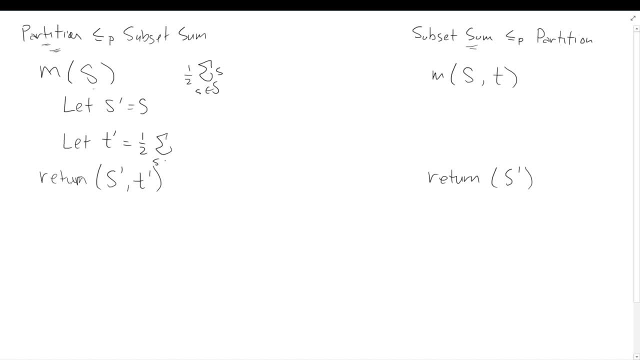 One half of all the S's in S And if we do that, then hopefully we can argue that we've got a. we've got a correct reduction here. Remember: what makes our reduction correct is that if we have a yes up here, we get a yes down here. 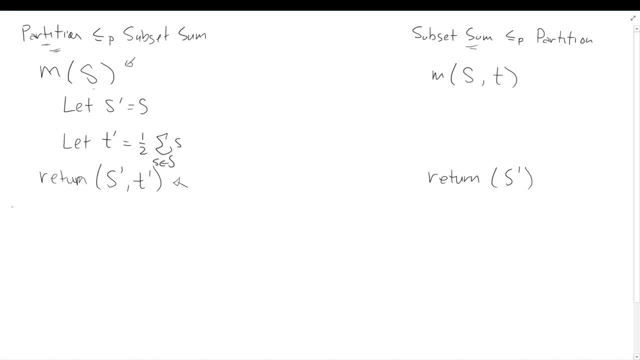 And if we had a no up here, we get a no down here. Okay, let's see if we can argue that. So we'll assume that S can be partitioned. We'll just assume that S can be partitioned into two sets with equal sum. 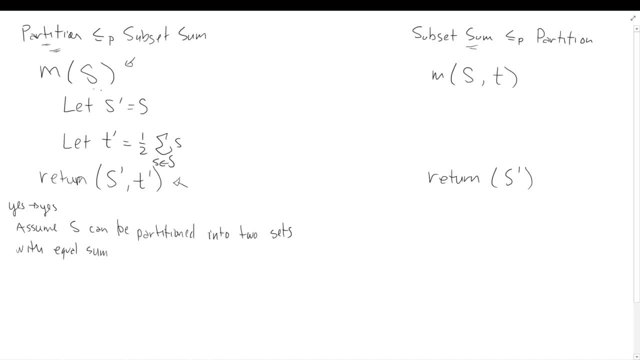 That is the definition of a yes instance for S. So let's now we need to argue that subset, sum, that our, our S prime will have a subset that sums to T, So or T prime. That's not going to be too hard because we can say each of these sets sums to 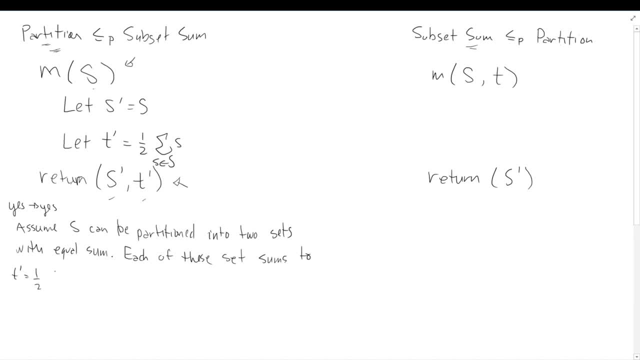 and I'm going to be explicit here. I'm going to say T prime, which is one half of all the S's in S. So S prime, which is equal to S, has a subset that sums to T prime, And that's what we wanted to argue. 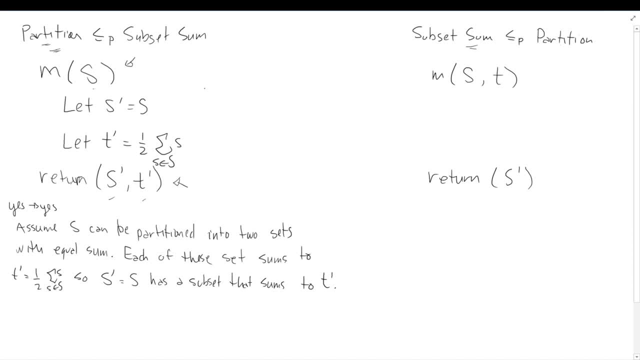 Okay, now we need to do the other argument. Now again, we can do that. no implies no, Assume there's none up here, therefore there's none down here. But I usually like to go backwards because it allows me to repeat the same argument. 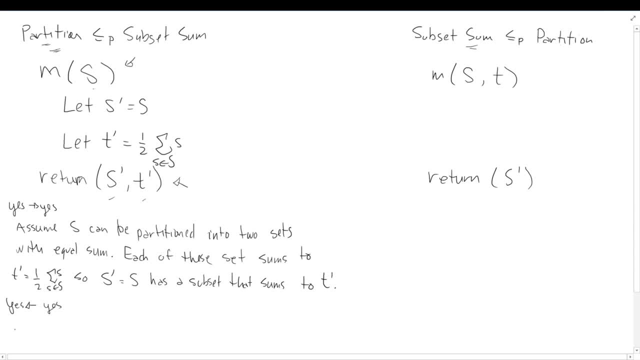 So now my argument is going backwards, So I need to start where I finished. Assume that S prime has a subset that sums to T prime, And at this point I'll just reference and say: well, this is going to be equal to all half of the S's in S. 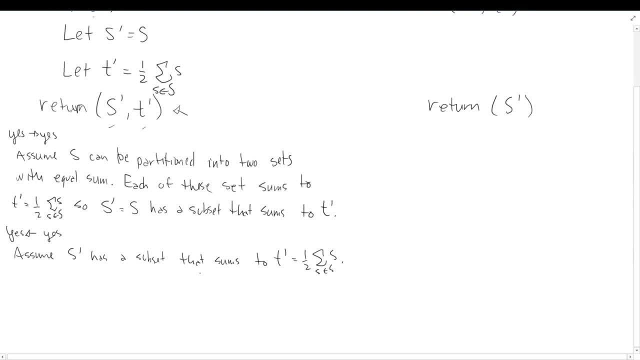 Half of the S's in S. Okay, so if I've made that, that's the S on the bottom side, I need to argue that we were yes on the other side. So this is saying that there's a subset. that sums to this. 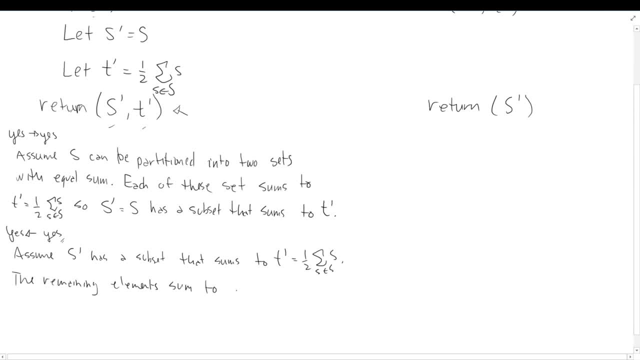 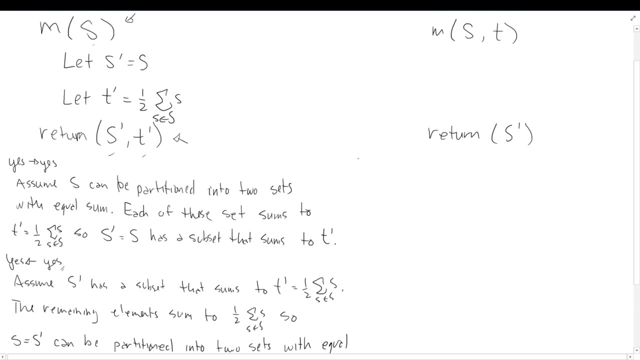 The remaining elements sum to the same value. So S, which is equal to S prime, can be partitioned into two sets with equal sum, And we're done. Okay, we're done that one, And in fact this reduction that we've created over here is actually kind of easy. 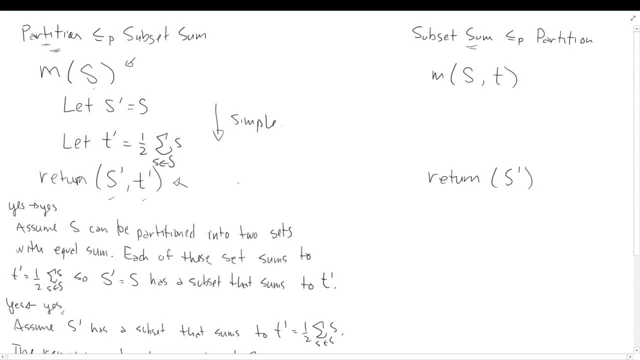 This is sort of a simple one. Okay, but what we'll find sometimes when we have two problems, especially two NP-complete problems like this? we're actually guaranteed that if we have two NP-complete problems, they reduce to one another. That's one of the promises. 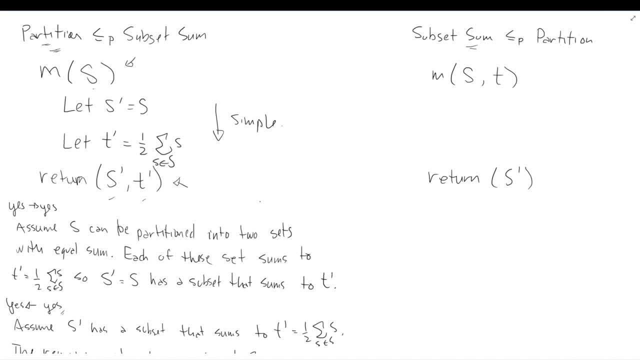 NP-completeness defines an equivalency class where every problem in that class can be reduced to every problem in that class. Now, just because we're guaranteed that that reduction exists doesn't mean that it's going to be particularly an easy one to come up with. 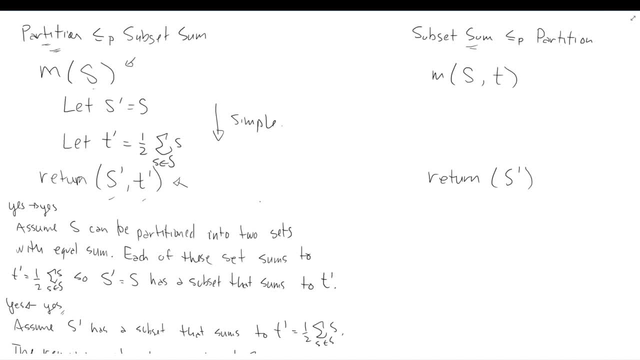 So in this case this was an easy one, And the reason is because partition is a special case of subset sum, So subset sum is more general, Partition is more specific. It's usually pretty easy to show that the specific problem reduces to the general one. 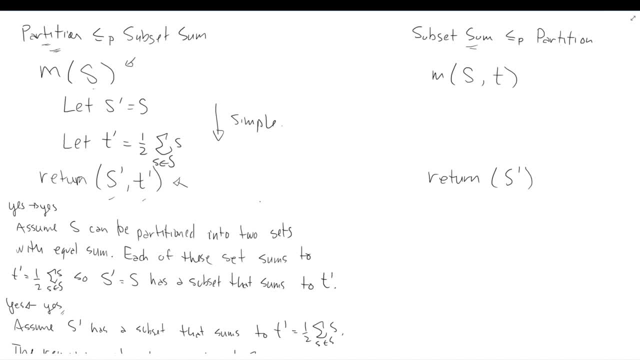 That makes sense. If you can solve the general one, you should be able to solve the specific one. But what this other direction is asking us to do now is saying: if you can solve the specific problem, then you can solve the general problem. 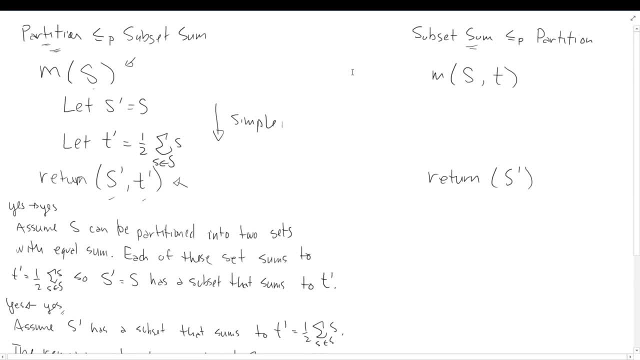 And that sounds a little bit harder. So again, an example of this is: say you know how to multiply by two, You multiply by ten. Can you use that to multiply by any number? Well, multiplying by ten was easy, So maybe multiplying by any number is harder. 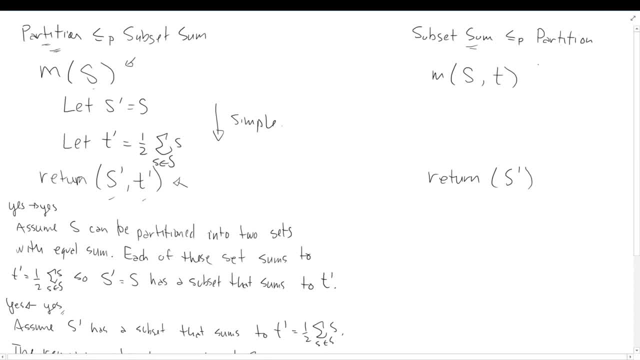 So this challenge here is saying: just because I can solve it for one possible value of t, one input value of t, can I solve it for any input value of t. So here the challenge again is a little harder. Here we had to come up with a t. 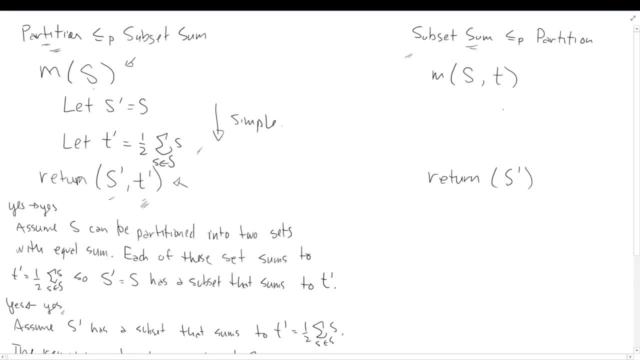 but that was just as simple as figuring out what t was equal to. Here we need to somehow build t into s prime, And actually to do that we're going to need a little bit more space here, because this is going to be not a simple reduction. 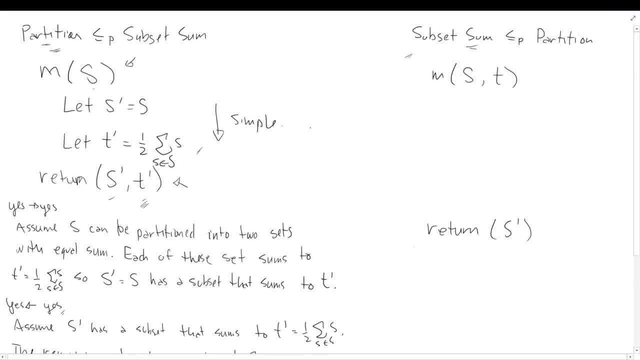 So I'm just going to give myself a little more room here, But I also want to think of a couple scenarios here, And to do that I want to draw a little diagram here. So imagine here what this is. So here, if we do the 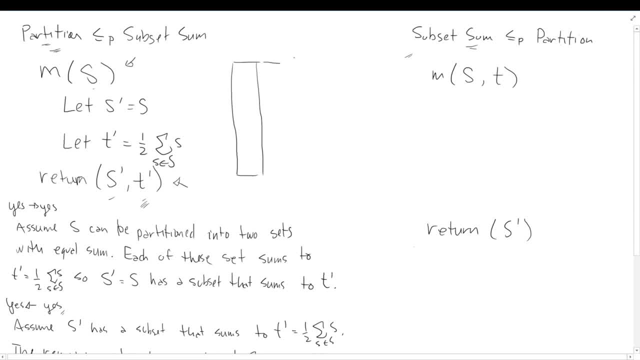 here. maybe I'll write it here- that this line here is the sum of all our s's in s Okay, Which means I could put a line down here which would be at half of that value, which was exactly this value down here, remember. 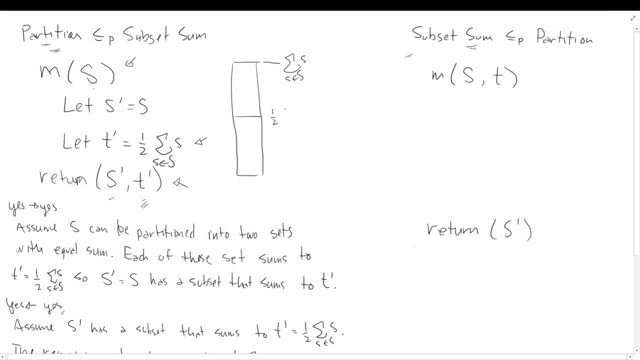 Now here's the possibility. If let's say, let's say our t, this is our t, this is our t, here we have a possibility. Our t could be equal to this line. it could be pointing right at this line. 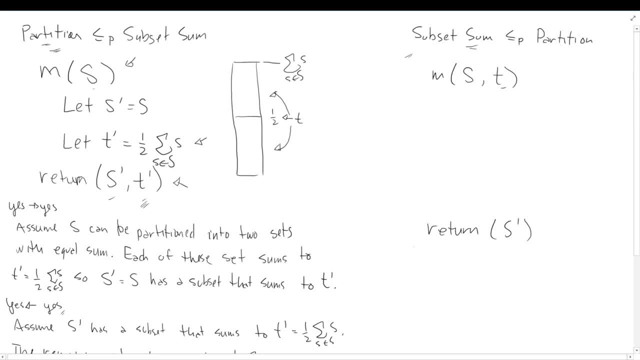 it could be above the line or it could be below the line, And we need to consider each one of those cases in turn And I'm going to do it easiest to hardest. So the easiest case is if our t is exactly equal to one half. 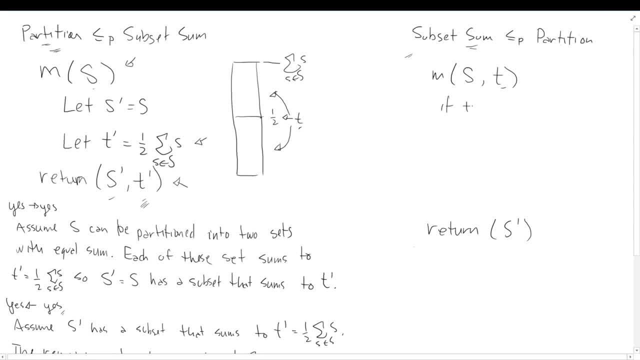 then we're actually done. So if t is equal to one half of all the s's in s, then we'll just let s prime be equal to s. We're done Because we got lucky. The input that we got for t was actually asking us if we could evenly split it in two. 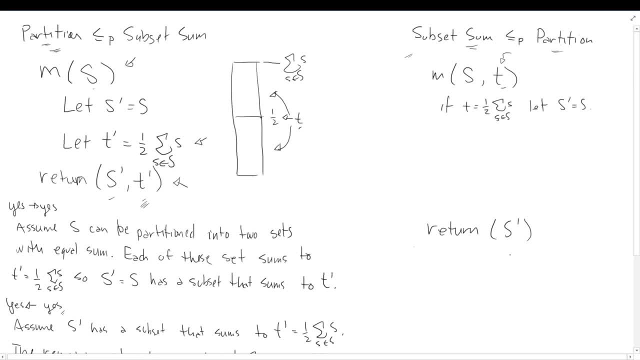 So since that's what partition does for us, we just ask partition straight up. But that only works for us when we get lucky, Only when our t was equal to one half. So now I need to consider one of my other cases, And actually again. 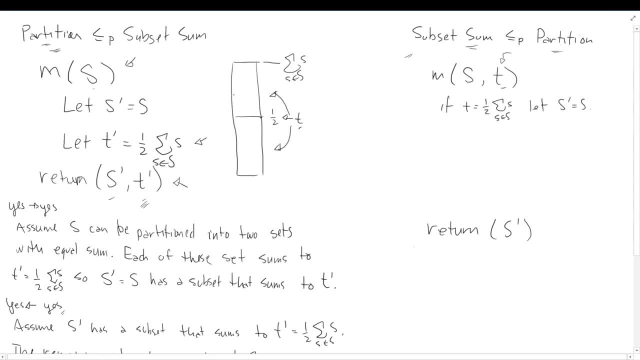 I'm going to try one that's maybe a little bit easier here. I'm going to assume my t is up here. It's above one half Okay. So I want to know if there's a subset that adds up to t. Now the way that I'm going to do this. 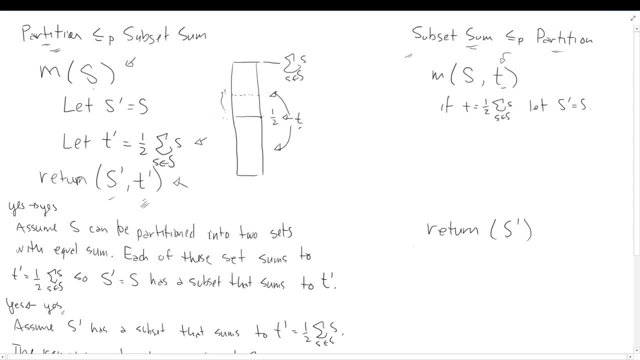 is. I can float this half line up here if I add some other element on Okay. Now, this extra element on that I'm adding here is one that I'm going to assume does not belong in the set of size t. It's just a bonus one, an extra element. 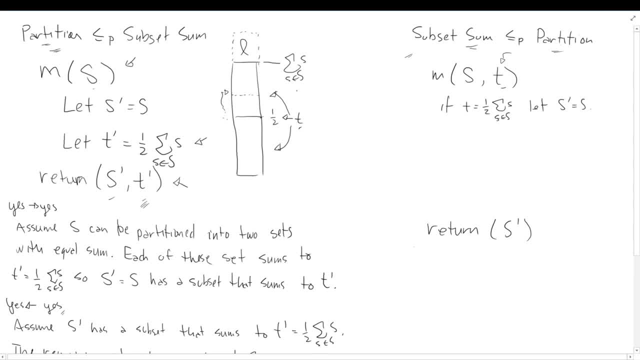 And I'm going to call it l here for a second. Now the thing is, I kind of want to solve for what l is equal to. Now, how do I know what I want to do that? Well, I want l to be big enough that this halfway point. 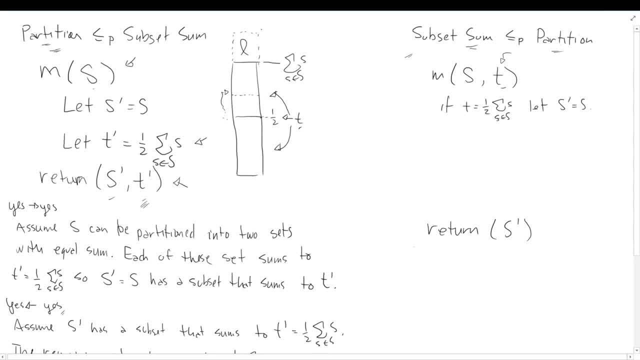 floats up to be equal to t, which means this should be 2t, Okay. Or another way of saying that is: we can see here what 2t is equal to is: it's this sum plus l. So I'm going to do a little scratch over here. 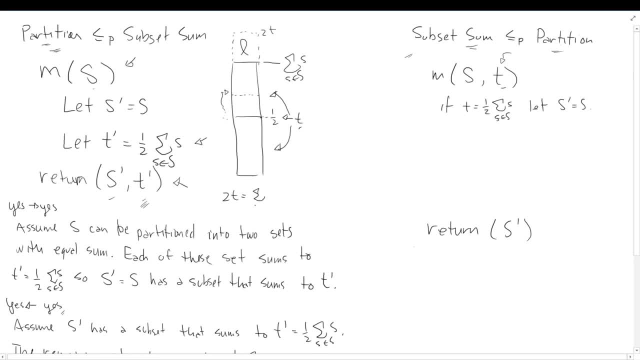 2t is equal to the sum of all the s's and s plus l, So that means it looks like my l. that's what I'm trying to solve for here. l is going to be equal to 2t minus the sum of all the s's and s. 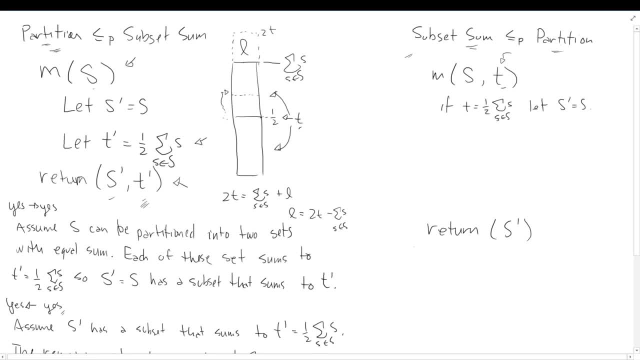 So by adding that l in there, if there was a subset that added up to t before, there will now be a subset that is exactly half, because now the total sum will be 2t. Okay, So that's our idea. So we're going to say: 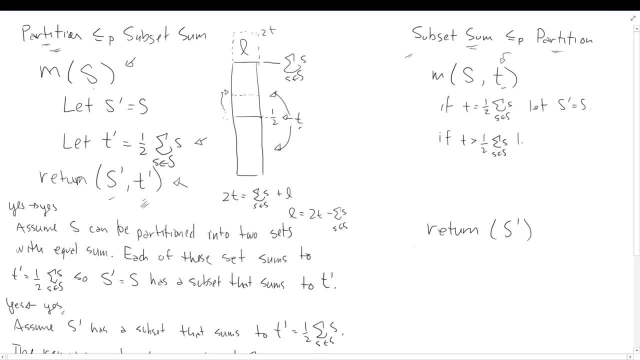 if t is greater than this value. now we're going to let our s prime still be s, but we're adding on this extra element l, which I'm just going to write its value here, which is 2t minus the sum. 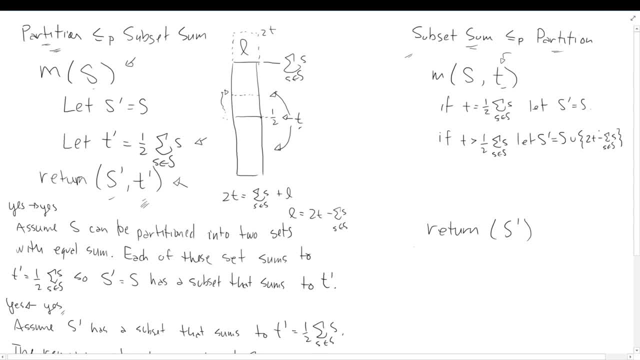 for all the s's and s. So this is a new element here and, if you want, you can call it l. So that leaves our last case. then What happens if our t is less than this value? Now we're down here and we got this. 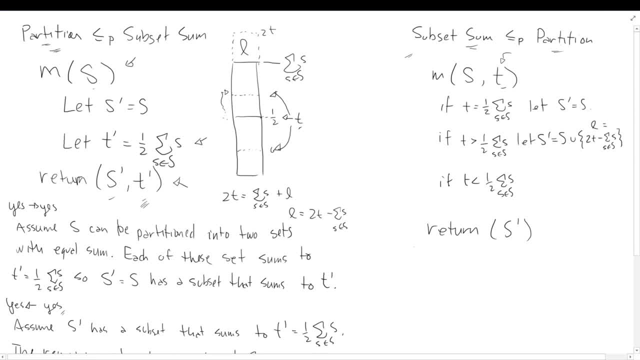 Okay, Now we have too many elements up here that are not in our set that adds up to t. This is the set that adds up to t, So now we kind of have to add in- I'm going to draw it on the bottom, sort of. 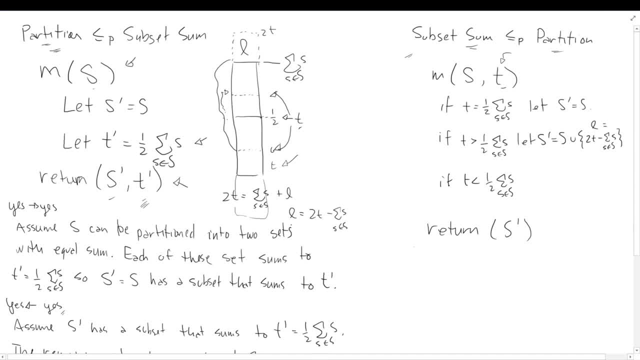 I need to add in elements that go into my set of t, Okay, So that we can again float up the t, really until it arrives at half, Okay. Now here's this. one gets a little bit trickier because when we add on this end on the bottom. 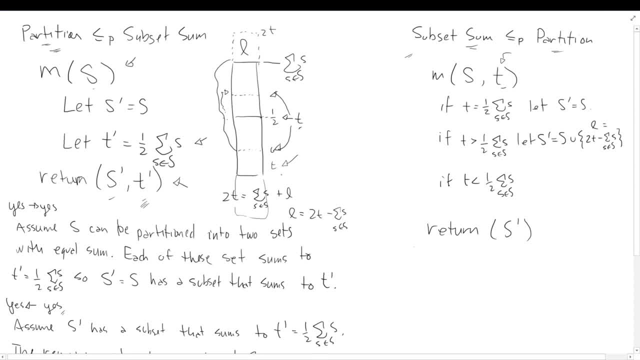 we're adding it in to the set of t, the set that adds up to size t. Okay. So again, we assume there's already a subset that adds up to size t. We add to it this new element, l. okay, and then that value should be equal to what? 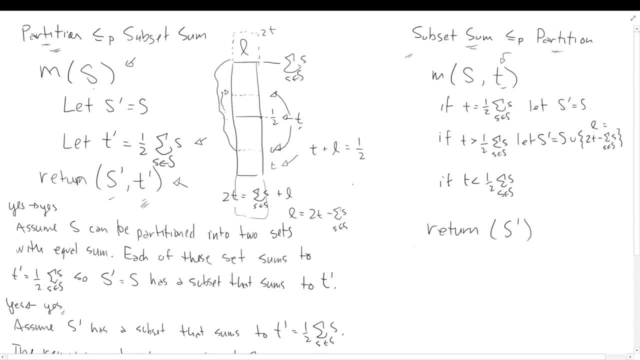 Well, that should be equal to one half of. well, whatever we're going to be adding here is still going to be the total sum plus our l. Okay, This gives us a slightly more complicated version to compute, but simply multiplying each side by two. 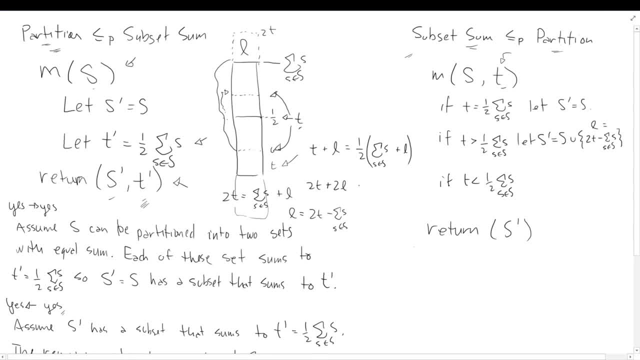 okay, we get equal to the sum of all our s's and s's again plus l. So now we can take the l off each side here, Okay, And then move the two t back over to this side. so we can see that in this case. 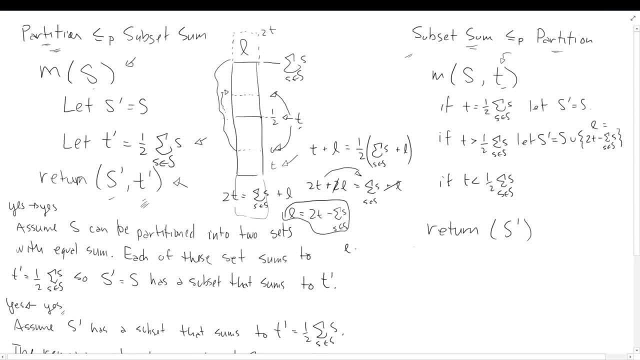 this was our first case here, okay, but in this case our l will be equal to the sum of all the s's and s minus two t. It's actually the inverse of this one. here We just reversed the terms, Okay. So here we'll: let s prime be equal to s union. 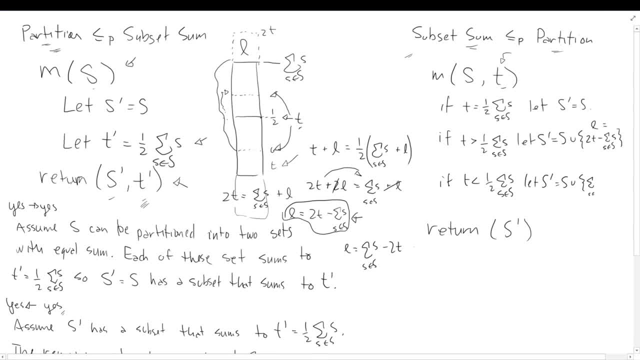 again another l, but here I'm just going to write its value, all the s's and s minus two t, So we're adding a new element in in each of these cases. Okay, So now what we need to do is we need to argue. 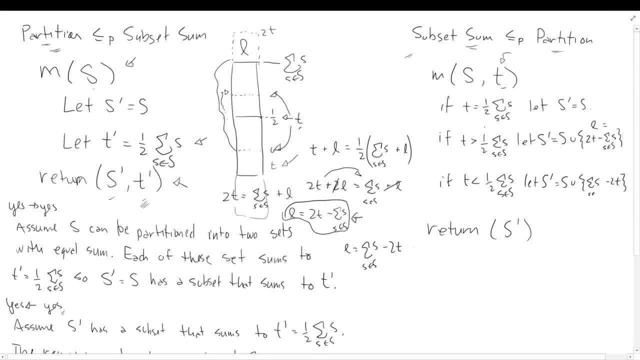 we need to build up our proof of correctness, And our proof of correctness is going to be, again, two branches. If we have a yes, then we have a yes. Okay, Let's see if I can get this started for us. So here I'm going to say: assume, 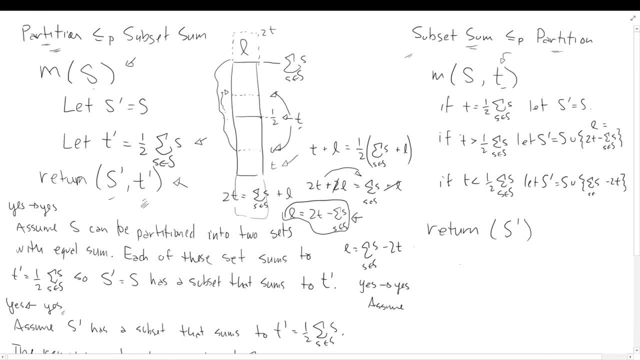 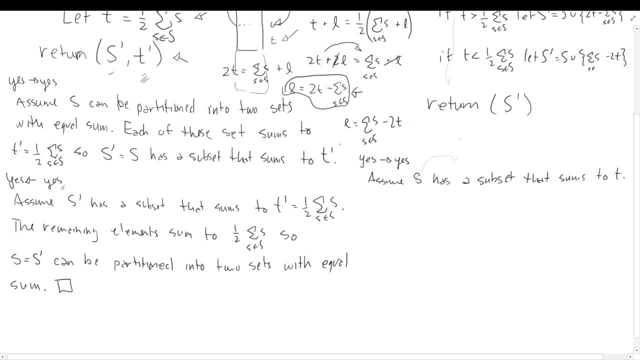 So, to start out, we're going to assume we have an s and a t, So we're going to assume s has a subset of size t, So we assume that s has a subset that sums to t. Okay, Now remember what we're trying to argue then. 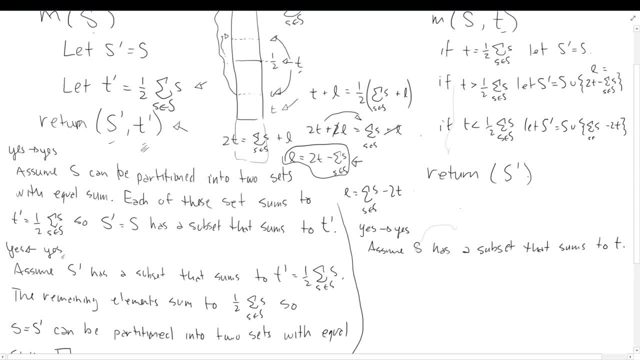 Okay Is that s prime will have a or s prime can be equally partitioned. can be partitioned into two sets with equal sum. Okay, Now to make that argument, then we need to know which case we are Okay. So let's start here. 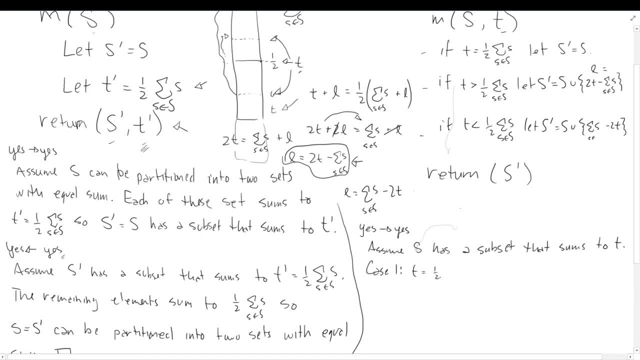 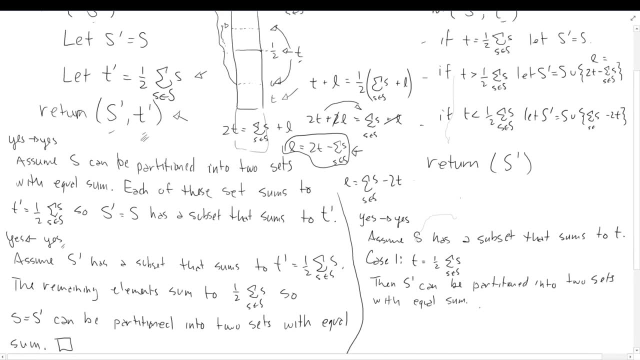 I'm going to say case one: t equals one half of all the s's and s. This turns out to be the easy case, right, As I already mentioned. this is easy because in this case where we got lucky, where t was already equal to half, 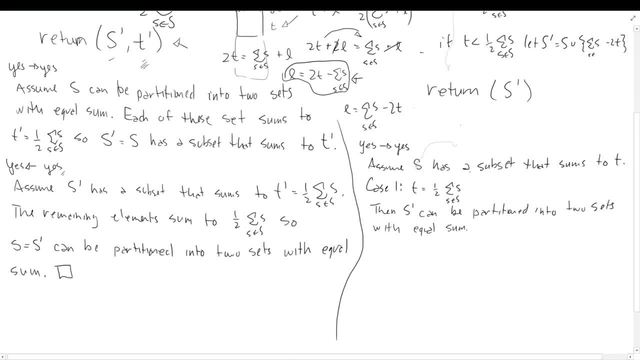 we didn't have to change anything. S prime was just equal to s. So since we already knew it had a subset that summed up to t, we knew that it could be equally partitioned into two sets. So we're done in this case. 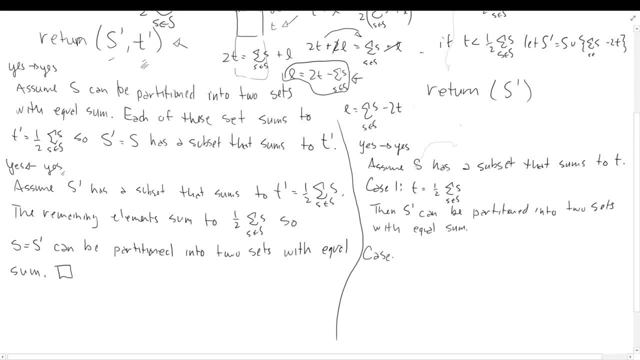 That was, remember, an easy case. So let's consider our next case here And we'll see where the algebra starts coming in here. So now we've got: t is greater than one half of all of our s's and s. Okay, 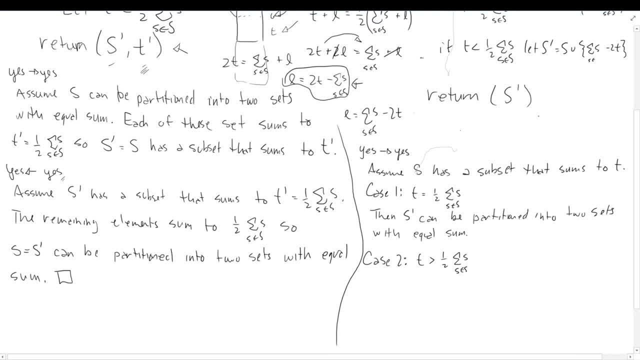 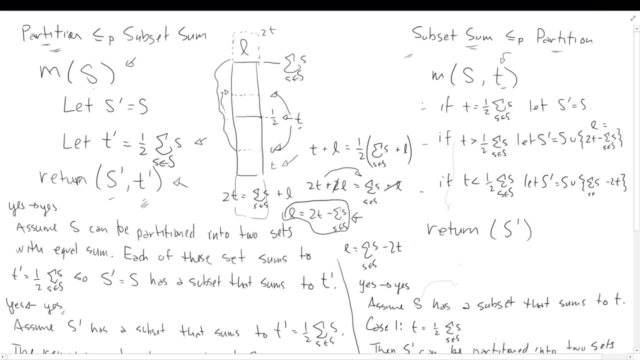 So let's just go back and see what is it that we were trying to prove, And I think my diagram sometimes helps me visualize or understand what we're trying to prove here. So now what we want to do is we still want to argue that it can be partitioned. 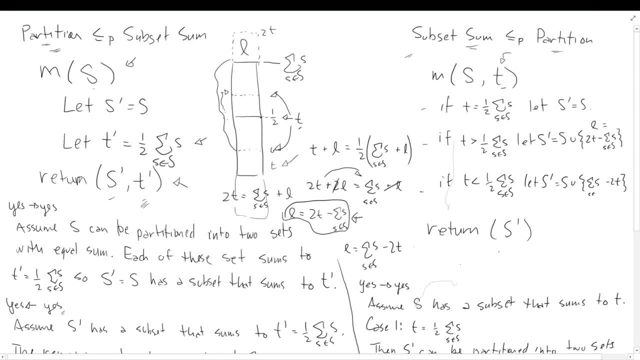 okay, into two equal sets. Since we know that it already has a subset that sums to t, we just need to argue that that is half of the total. Okay, So let's see what the total is. So I'm going to write this as follows: 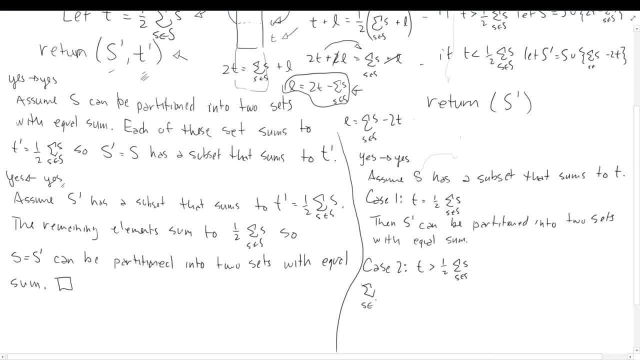 I'm going to write it as the sum of all the s's in s prime. Okay, This we want to be equal to two t, because we already know there is a subset that sums to t. So this is equal to what? Well, when we looked at this case, 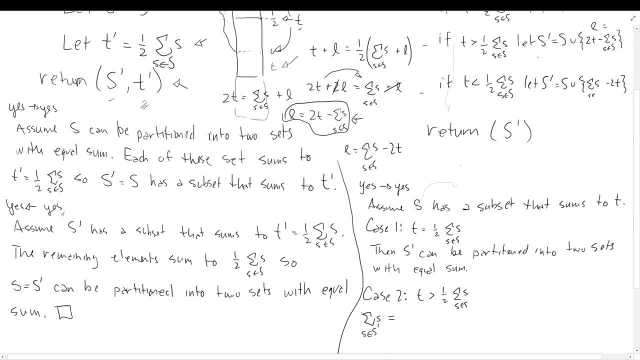 let's look at this case here. our s prime was just our s plus this extra one, So I'm going to say that this is equal to the sum of all the s's in s right, adding up all these ones plus our extra one. 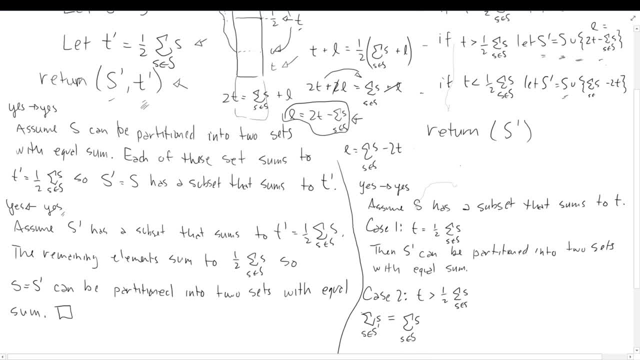 we're actually in this case sorry. So adding up all these ones and then plus this one, So we get plus two t, minus the sum of all the s's in s, We can see that these two cancel out. So this is equal to two t. 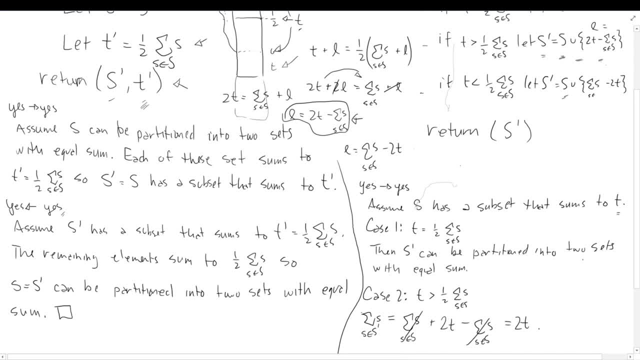 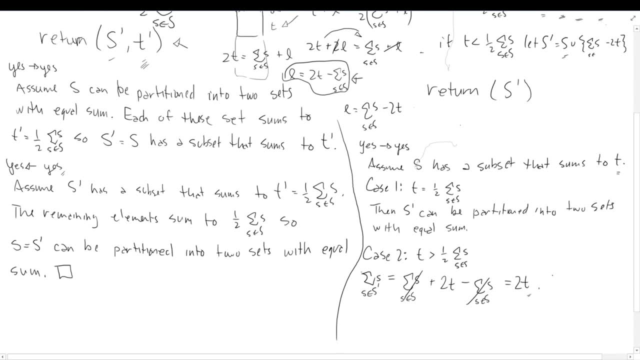 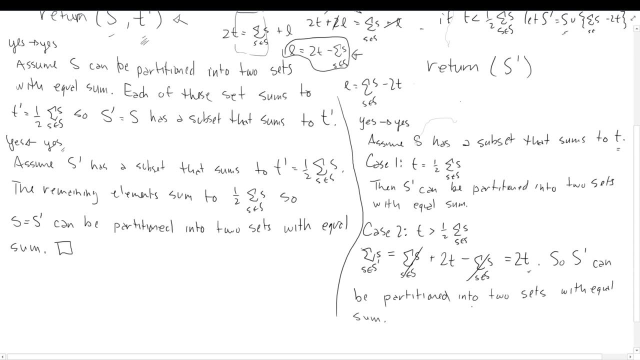 So, since there was already a subset that sums to t and our new set s prime totals to two t, there must be, so s prime can be equally partitioned. Okay, With two sets with equal sum, All right, So again. 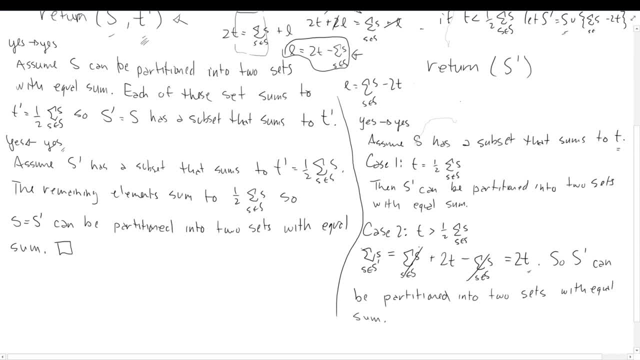 we just argued in this case that we, because we've increased the size of our set to two t and we now know that we have a subset that sums to t, that therefore we must be equally partitionable. Okay, That leaves us with our last case. 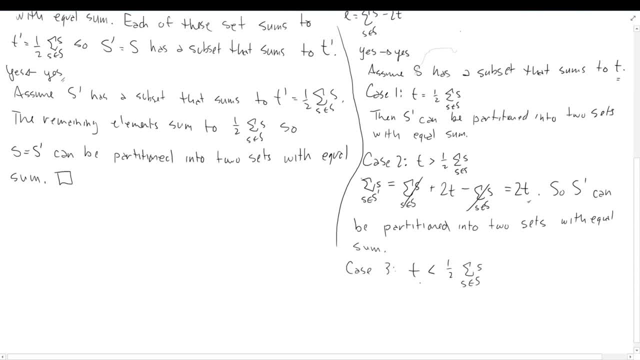 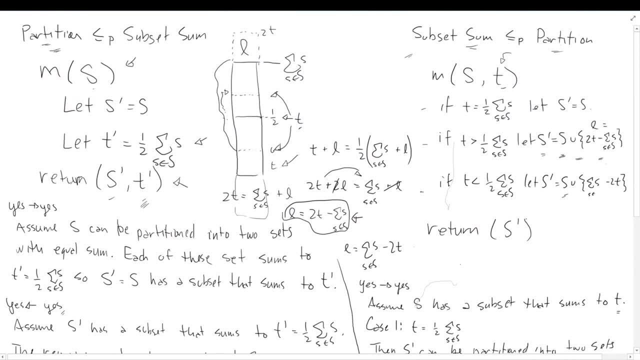 Let's try our last case here. So our last case was when t was less than Now. remember, in our last case we still added in this new value, but the new value was supposed to belong to this set. that sums up to t. 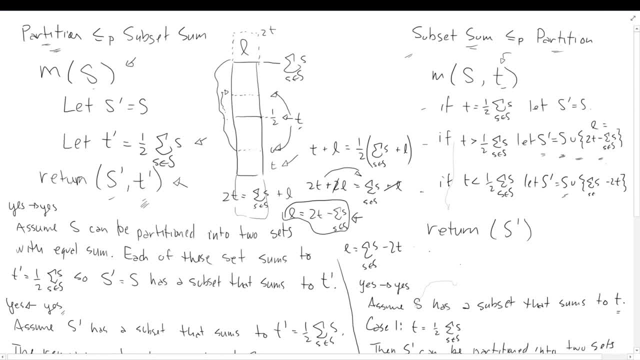 Okay, Maybe another way to think of this is sort of this is the parallel case, but where we maybe have a set that adds up to the sum of all the s's in s minus t, That one would be larger. Okay, So again. 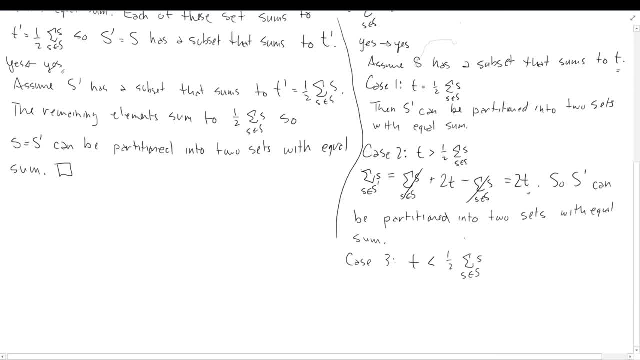 we still need to. we need to still consider this case. But now what I want to do is we're going to say our set is of size t plus l, So let's see what the total set is going to be equal to. So again, 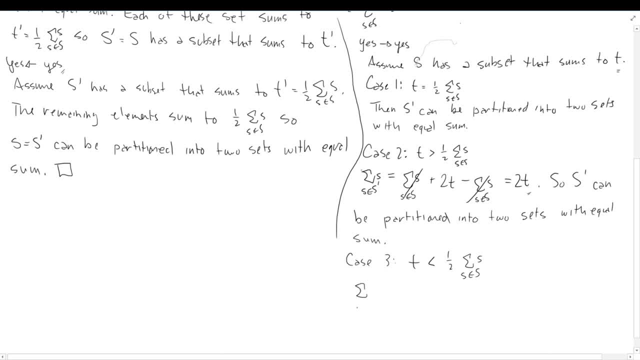 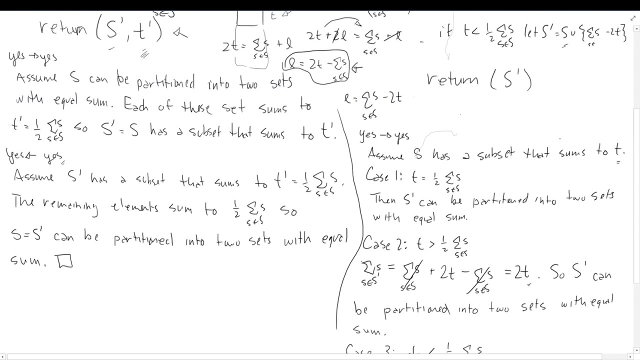 let's look at our sum for all of our s's in s prime. Okay, That's going to be equal to same as before: Our sum of all of our s's in s, plus, like we had before, our new element. but our new element is different this time. 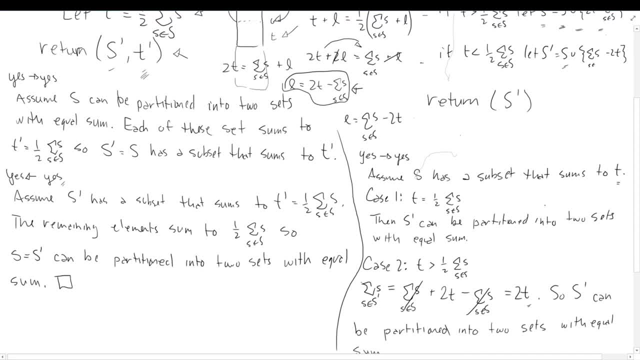 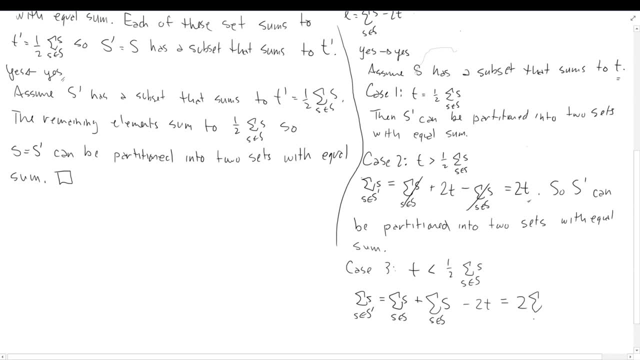 It's this one here- the sum of all the things minus two t, which altogether we'll see, We can rewrite as two times the sum of all the s's in s minus two t, Or if we wanted to, we could factor the two out of there as well. 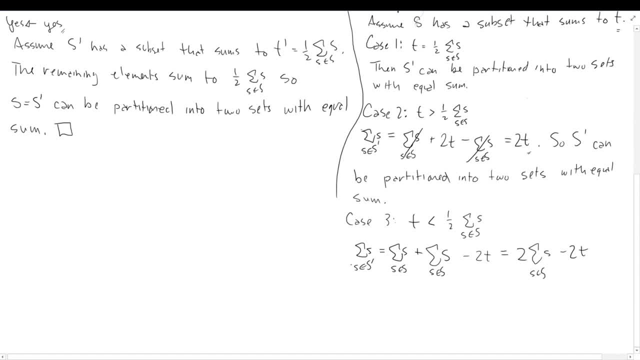 But let's see. So this is telling us how much all of our set is Okay. And now what we can see is we can take the set that's of size t, that we know exists, And we can add on it to our extra value l. 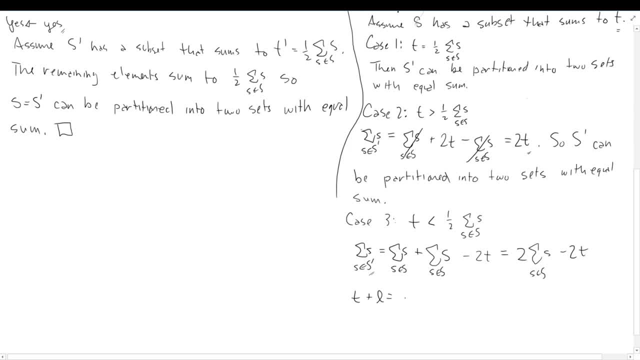 Now our extra value was just this sum here as well. So we got t plus this sum here, All the s's in s, minus our two t. Okay, Which will give us. well, look, this term stays the same. s is in s. 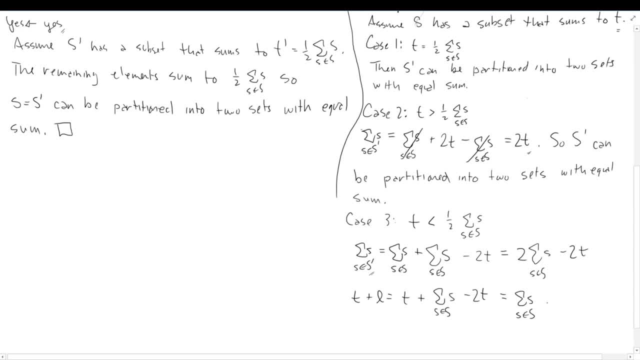 t, or two t minus the two t. sorry, plus the t will just give us a minus a t. Okay, Now notice that this one here is exactly twice, two times this one here. So this is the total Size And this is the size of our subset. 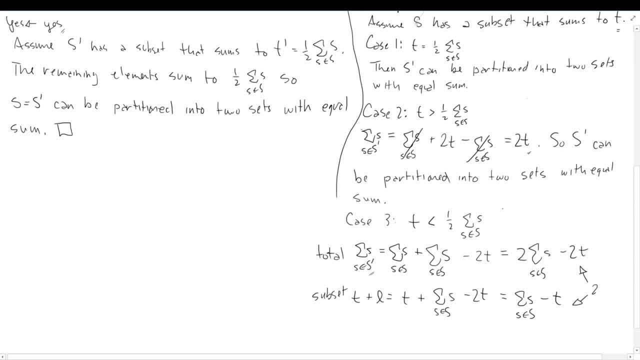 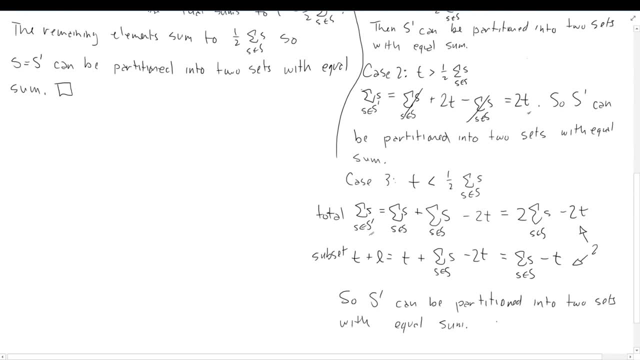 So once again it's half as big means once again we can argue that we can be partitioned into two sets with equal sum. And that concludes this branch of the proof. Now, as you can see, this branch of the proof is pretty long. 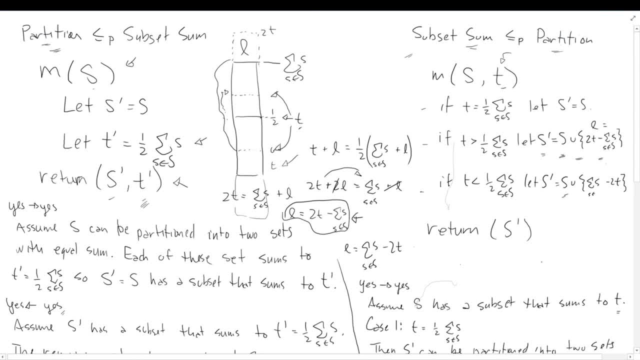 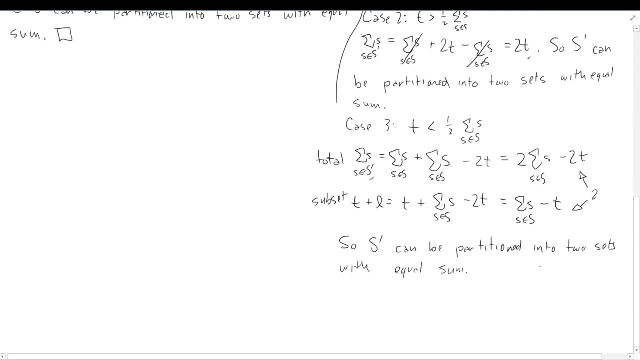 And at least for the purpose of this video, I'm not going to do the other branch because it's just a repeat of the same arguments, Just in reverse order. So I will leave that as an exercise. It will still need the three cases. 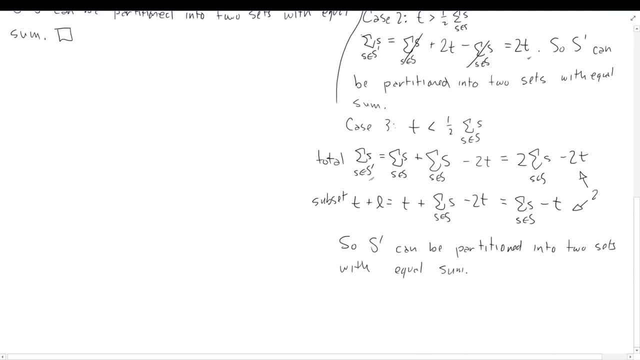 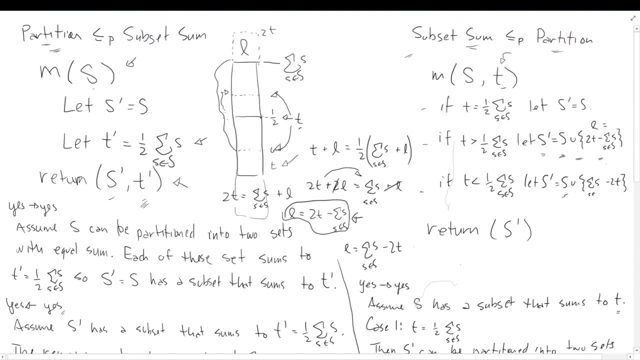 But it's just going in reverse order And the math will be the same as well. But this case, the one reason I wanted to bring up this reduction and take a closer look at it. So two points, I guess One is when we have two problems like this. 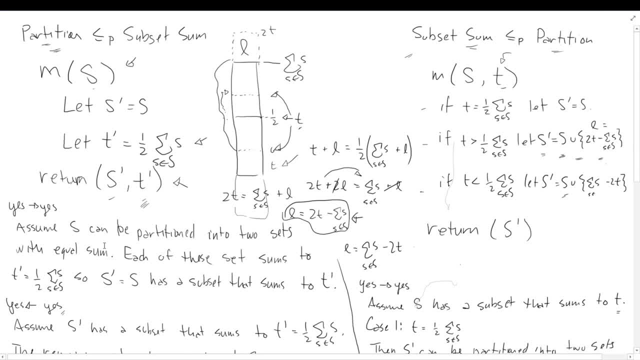 one reduction could be easy. So the one on the left here was easy, The one on the right was more challenging. And then the second point I want to point out that I wanted to make is that these extra elements that we added, that I was calling L. 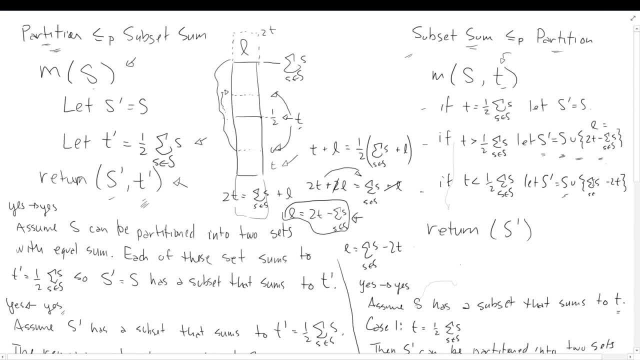 these extra elements we created to have a specific property so that we could make the reduction work. now, In a lot of the proofs that you might encounter online of other reductions, and this is certainly true of a lot of the proofs in the Gary and Johnson book,